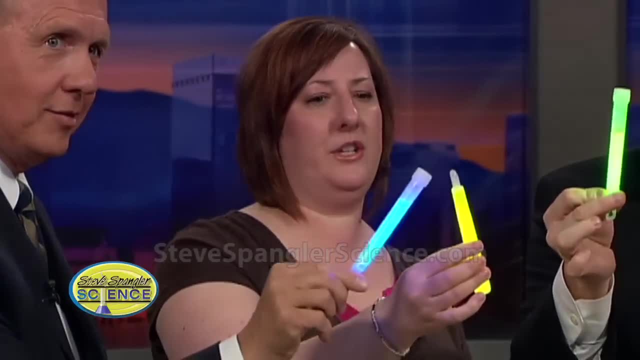 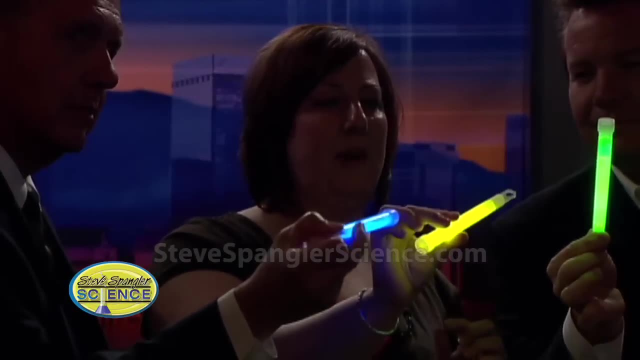 reaction that's happening here Now. sometimes, when you have a chemical reaction, you'll see things like: the color will change, things will bubble, there might be heat, but these are nice and cool. This is chemiluminescence, which means that it's releasing energy in. 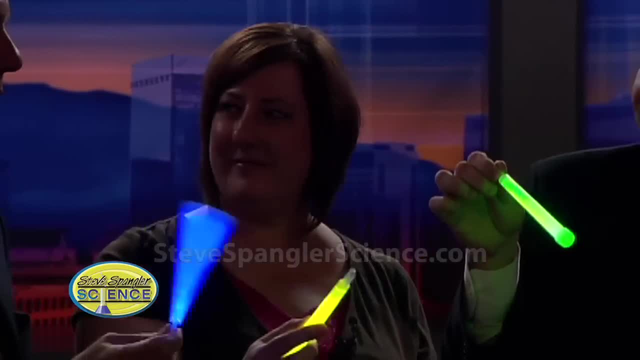 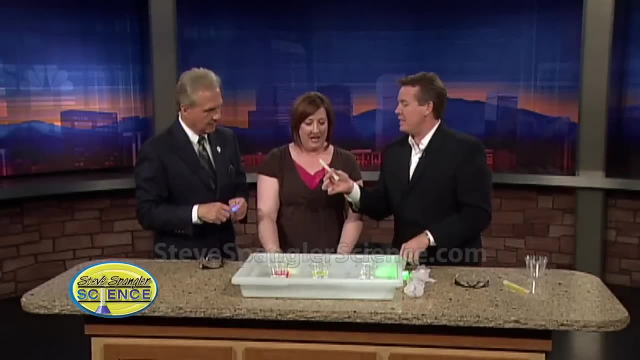 the form of light. That's cool. That is cool. You do see them everywhere, Absolutely everywhere, And the kids think that they're battery powered, and of course they are not. There's two chemicals inside and she actually cuts it open to show you. 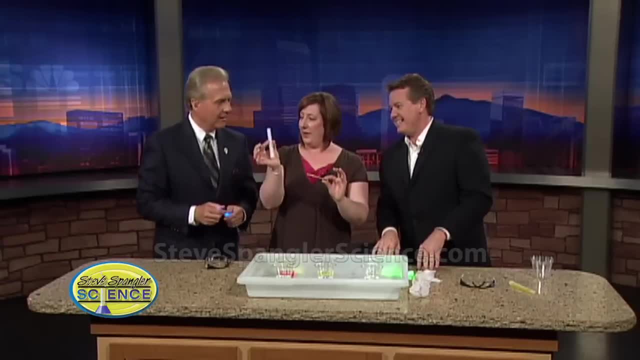 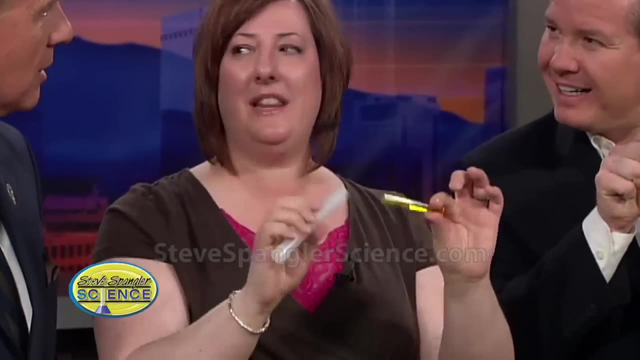 I bet you've never seen this. Look at this. Here it is. There's one chemical inside this ampule and one chemical inside this ampule, So that cracking sound that you hear is actually that those two ampules breaking. It's kind of like Da Vinci code, where they have the 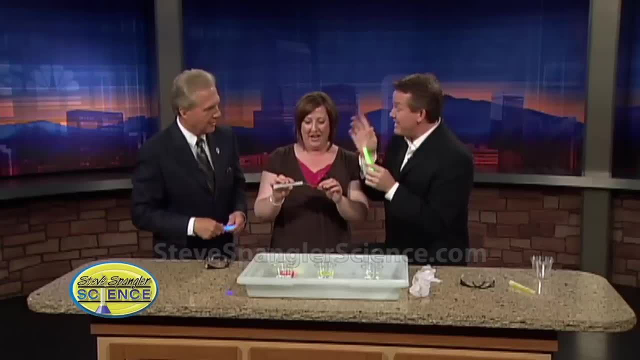 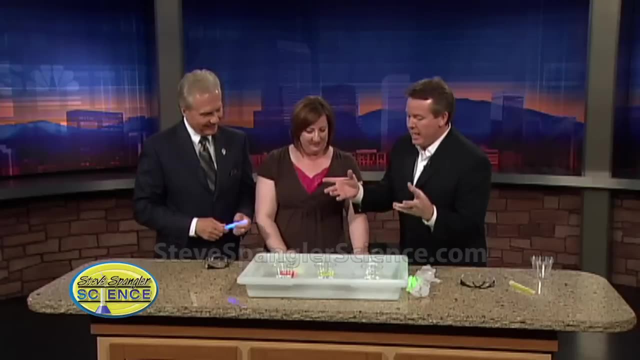 thing and if they broke it, it dissolved the papyrus and all that. I don't think this is on Da Vinci code, but that's nice. So here is the cool thing is that in China they will take these liquids here Instead of a unity candle for a wedding ceremony. they actually 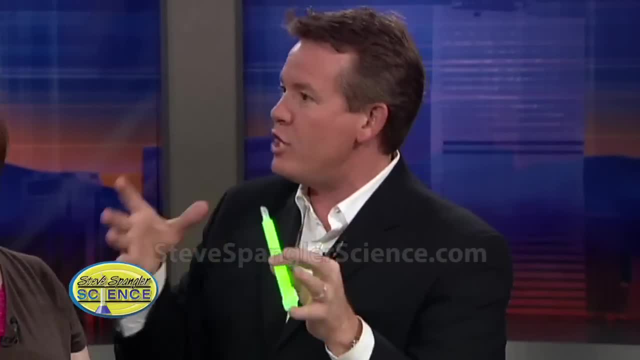 take the two liquids and they break it open. So they break it open and they break it open, So you can take the two liquids and pour them together on the altar. It's kind of a new generation thing. So look, here are the actual liquids. So, Mark, put on your safety glasses. 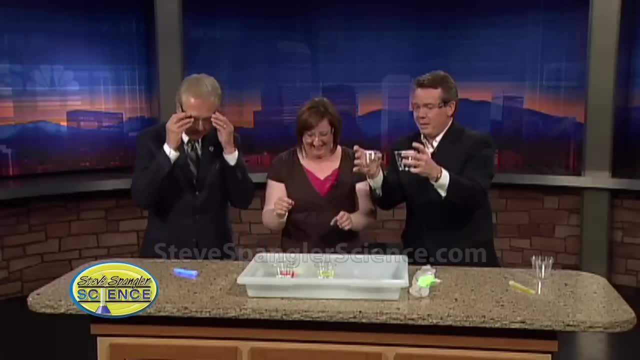 Safety first. She has two of us to blow up or set on fire today. Alright, so pick up your little mixture. These are mine, A two part mixture, right? So now let's do this. Let's dim the lights first and then. 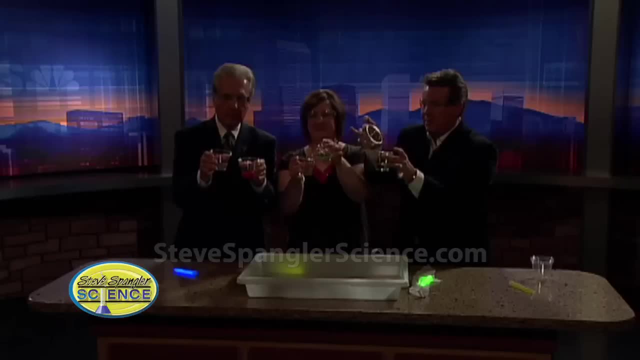 as we mix. if you stay on that white chart and as we mix you start to get to see it glow, Ready, Mix it in There, they go Nice, Back to the other one. Oh, sure enough. Oh, look at that. 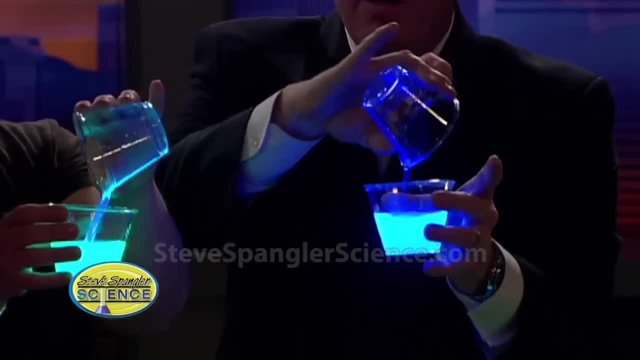 That's so beautiful. So we get this liquid that glows, Now bioluminescence. Bioluminescence would be like a firefly, is that right? That's correct, And we don't have many fireflies here in Colorado. 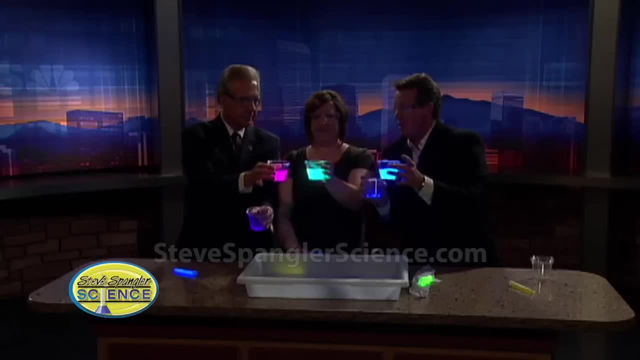 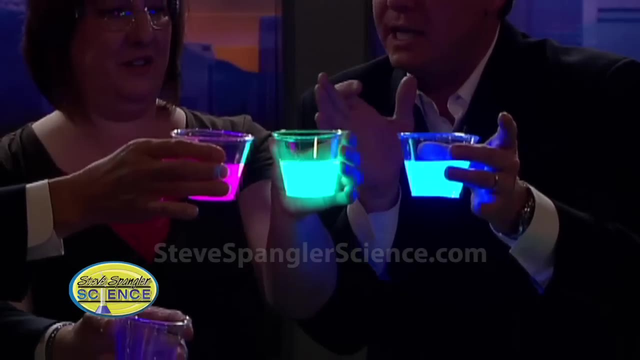 So here's what we were thinking. Look at what we have are the primary colors. Mark, We have red, green and blue. Colors are the right. Roy G Biv, You are good, Thank you. So this is for no yellow, of course, in science. so it's red, green and blue. 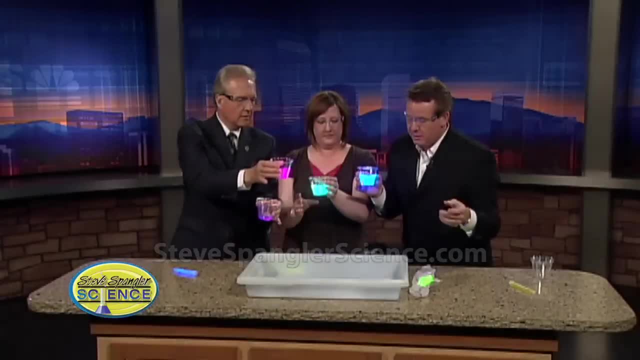 So here's: what we're going to do is bring the lights back up again and I thought if you mixed them together could you make white. So here's our handkerchief. So our handkerchief goes like this, and we're going to kind of lay it here and now. we just